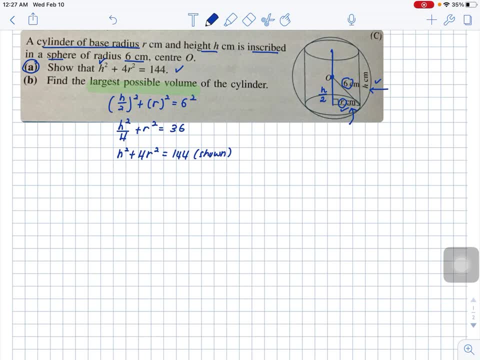 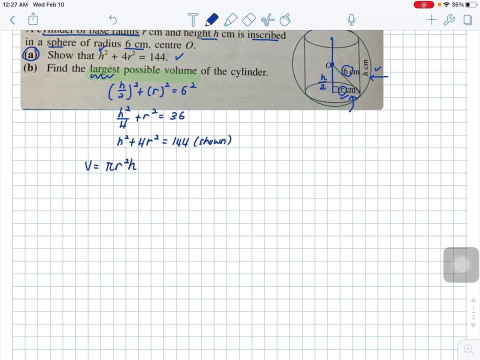 I have to find either one, So which one you want to find? So let's begin by writing the formula of the volume. Volume of a cylinder is pi r squared h- See, look at this word: largest volume. So this largest is the largest volume of the cylinder. So this largest is the largest volume of the cylinder. 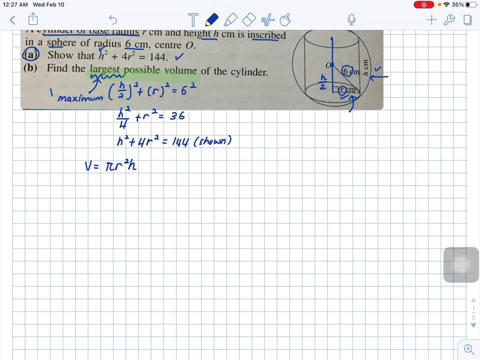 This is simply means the maximum volume. I'm looking for this one. Since you know that this is an optimization problem, you should think of differentiation. You know, at maximum or minimum point the gradient is going to be zero, Right, so we're going to use that. Now, will I be doing dv over dr or will I be doing dv over dh? 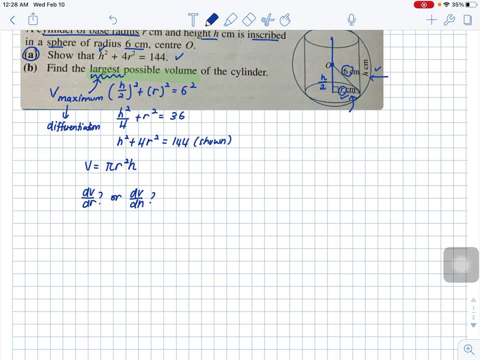 Which one? That is the first question. Second question: you look at this: your volume is being expressed in terms of both r and the h. So you should not have two variable now. You can only have either r in your volume expression or the h. So this is pretty simple. Now you will know the reason of. 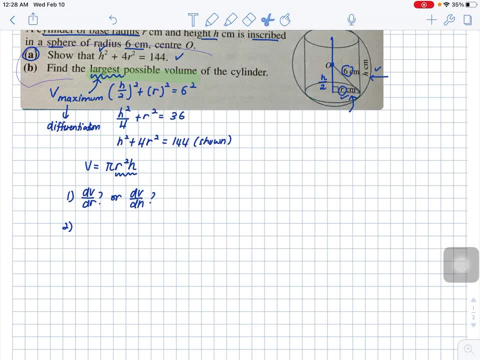 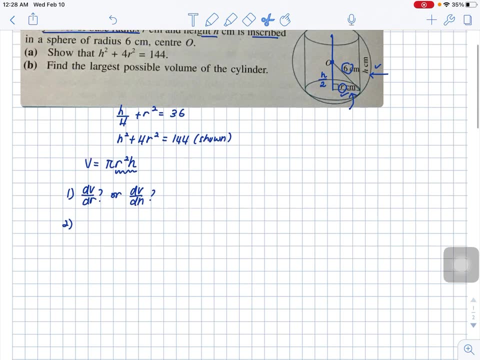 having the part a. You know it's a guided question. Okay, in part a they already help us By asking us to show h squared plus 4, r squared equal to 1 4, 4.. Okay, now you substitute. you should be able to express So pi now which one you want to change, which is easy to do. You look at this. 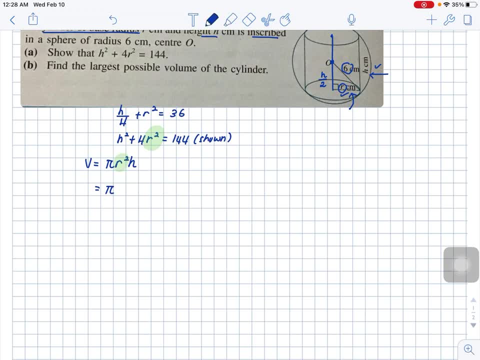 you have a r squared here and this is a r squared, So I think I'm going to make a volume in terms of h. So let's rearrange. You're going to get 1, 4, 4 minus h squared over 4 and then h. Now you pull out all the constant pi over 4 and then you take your h and then you. 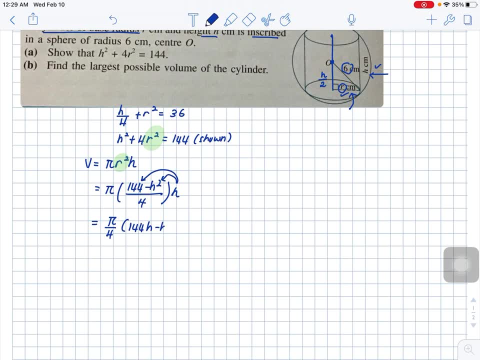 individually multiply. Okay, done. Now let's say, if you are not doing this approach, you want to make v in terms of r. You can also do that, but it will look a little tedious, So you make h as the subject now. So 1, 4, 4 minus 4 r squared. 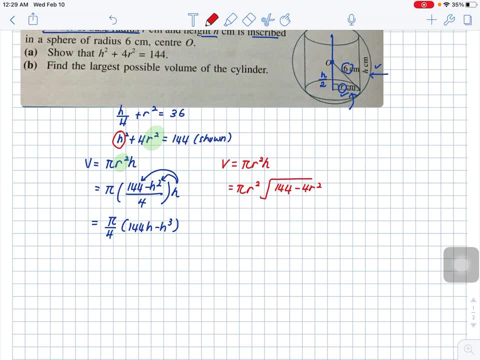 you will go and square Square root And of course we know h is greater than 0. So you don't have to worry about the plus minus, It's always plus. See, this looks a little tedious, So I think I like the blue method of. 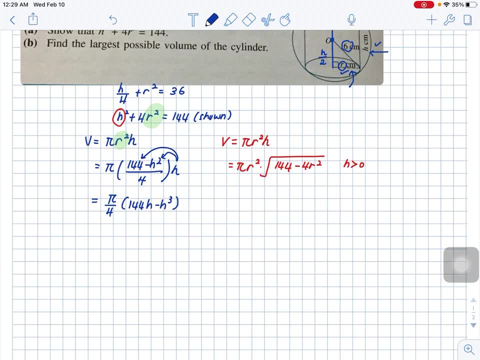 doing Okay now. So, as I told you, I'm looking for the maximum. So you do d v d h equal to 0.. Let's differentiate now. So when I differentiate what will happen? it's going to be pi over 4.. 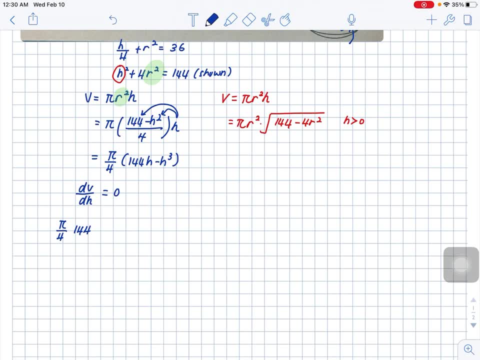 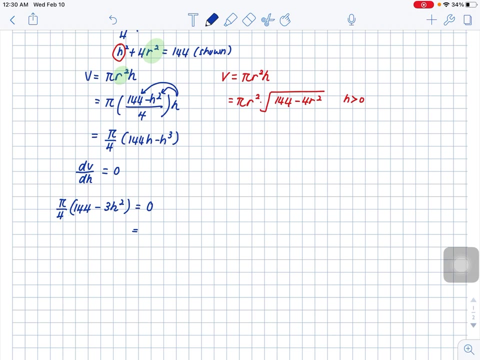 1, 4, 4.. And then pi over 4 minus 3, h squared, I'm factorizing the pi over 4.. The constant is not affecting your solution: 0 divided by pi over 4, it's 0. So leaving you with only this. So you: 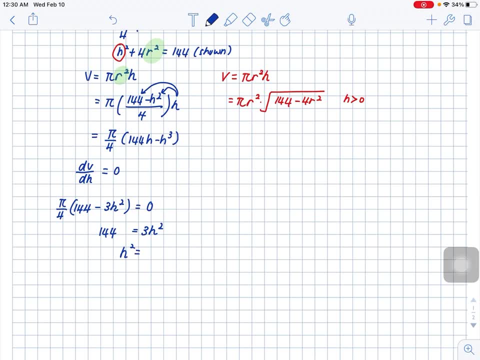 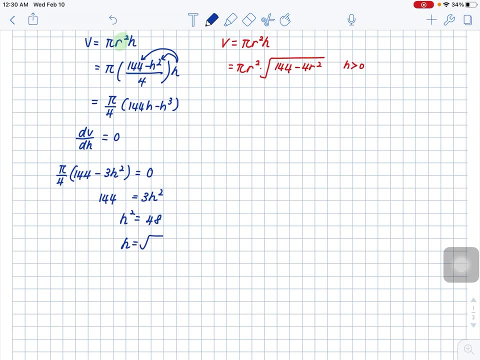 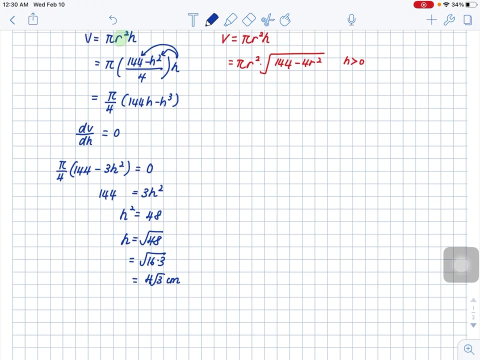 find the h squared centimeter. Now you can just use calculator and then you can express h in terms of decimal. So it's like you need the height to be 6.928 in order to get maximum volume. So if my h is, 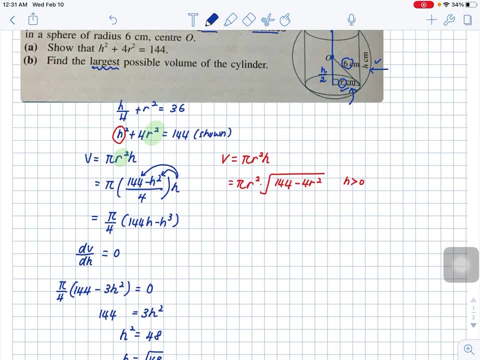 6.928. what will happen is that I'm going to get maximum volume. So if my h is 6.928, what will my r be? So you can substitute back into this. You will be able to get your r value. Okay, let's. 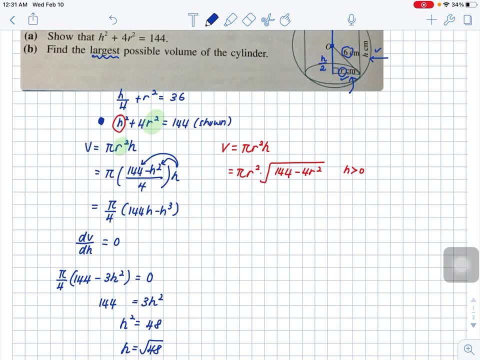 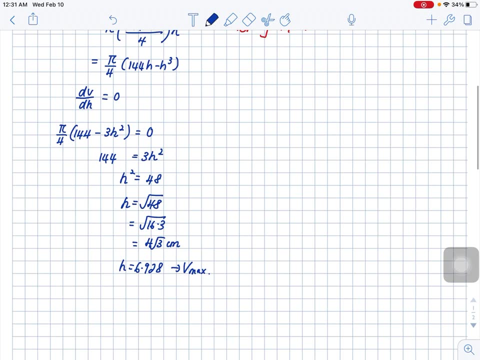 check. This is just extra, Let's see what happens. So your r is 2, search 6.. You can calculate on your own and that is like about 4.899 centimeter. So when your r and h is in this manner, 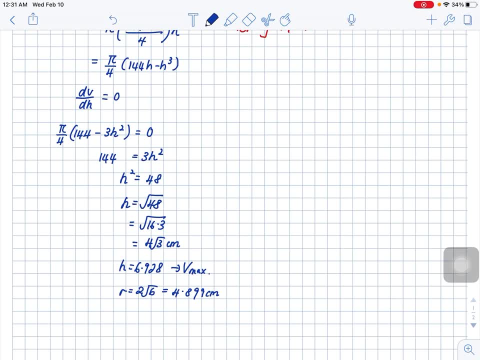 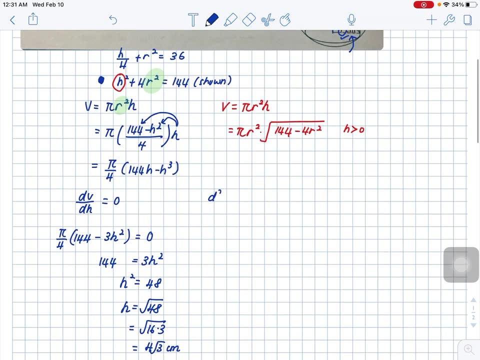 Theoretically we're going to get the maximum volume, But am I very certain that I will get a maximum value? So you have to check. How do you check? You do the second derivative, You differentiate another time. So we do it from here: The constant Differentiating constant, I get. 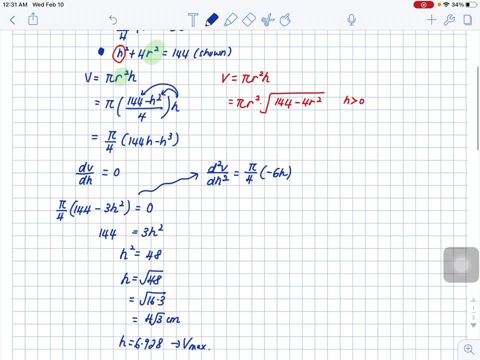 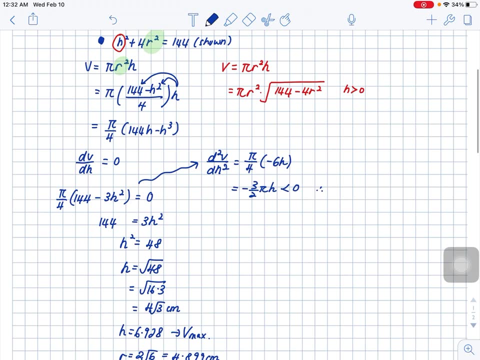 nothing So negative. 6 h So negative: 3 over 2 pi Height. Height is always positive and I know it's going to be less than 0. Therefore, you know, for h equal to 4, search 3. your v will be maximum Okay. 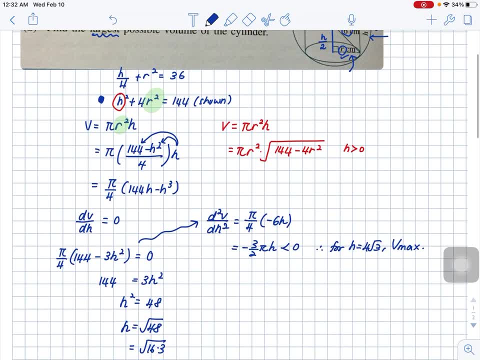 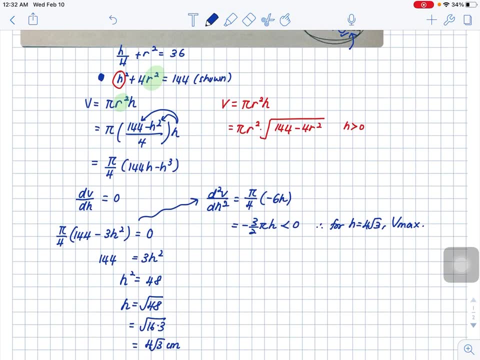 let's try to imagine how it's going to look like. And, of course, the question is asking you to find the value of the volume itself. So the h is not sufficient, The r is not sufficient, So we need the v. What you can do, you go here and substitute your value. 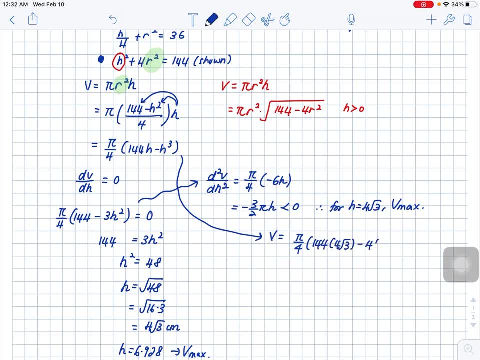 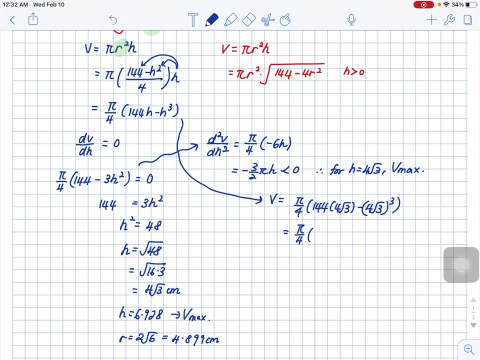 If you want to be nicer in your answer, This is typically 4 times by 4 times by 4.. And then you have a search 3. Search 3, and another search 3. Giving us 192 search 3.. So that is 96 search 3 pi. Let's see it in form of decimal so that we will be able to visualize. 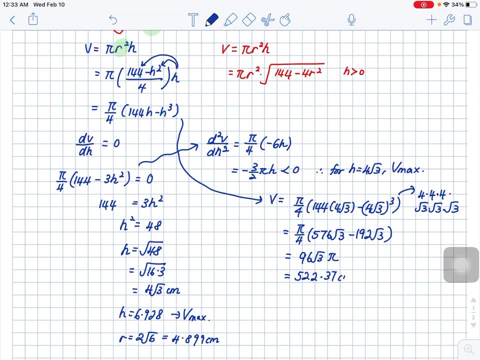 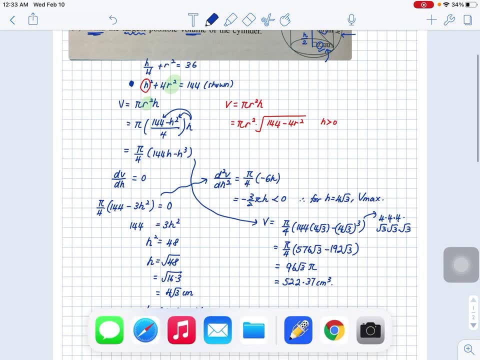 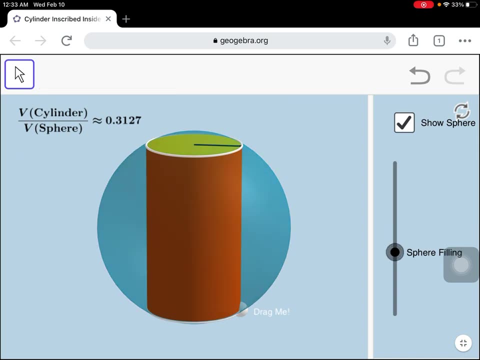 better. 522.37 centimeter cube, See, this is the highest optimized volume you can ever get. So this is the cylinder And you can see the cylinder is inside. Now, what kind? what are they asking? See, they are asking about the volume. You can imagine volume in the sense of how much water you are. 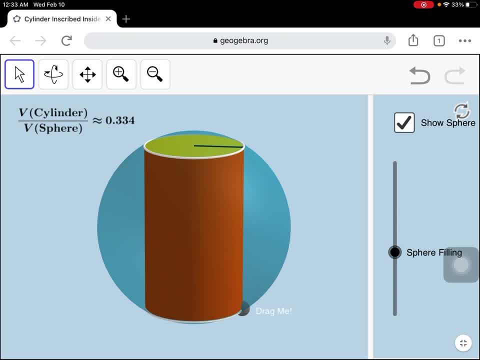 pouring inside the cylinder The amount. Okay, Then it will be easy. So when the r value is small, Look at this. When the radius is small, you are getting the orange shape. The cylinder is large. So when the r is a little bigger, then it goes this way. So the question is asking: find the 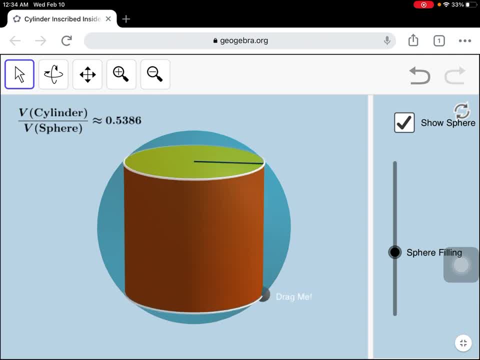 maximum volume You understand, Or you can even try this on your own. It is like an illustration. You can toggle around. You can use George Yipra to see this. I hope you see the benefit of solving the problem.